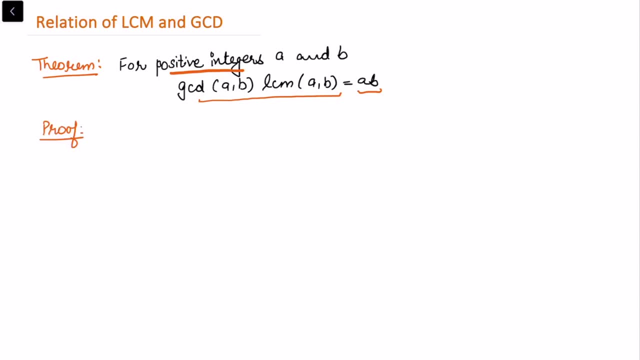 I've considered the two integers as positive integer. Now let us do the proof of this theorem. and for the proof, let me to start considering from the gcd. So let d is equal to gcd of a comma b. So considering d as a gcd. So, by the definition, when d is the gcd of a and 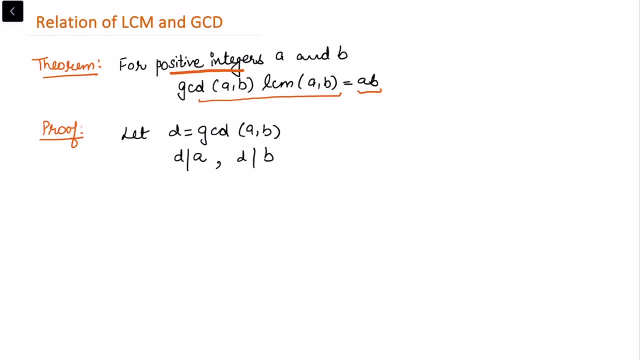 b, d must divide d and d divides b. and because d divides a and d divides b, So I can write a as multiple of d and also b as the multiple of d. So for some integers r and s. So for r and s. 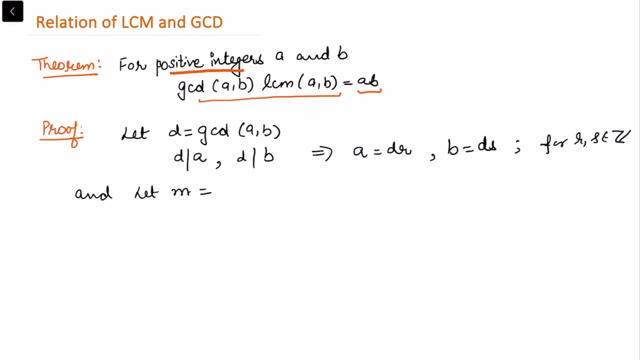 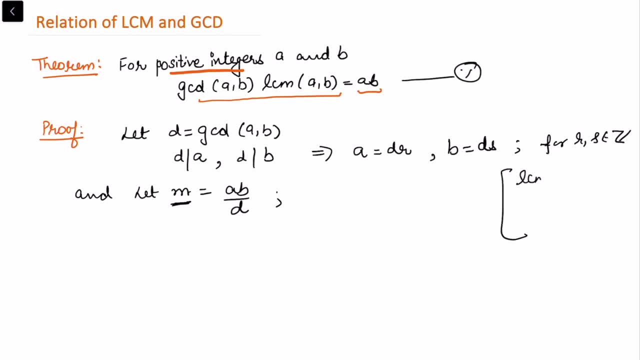 let me to call this as one. What we have as an expression, we have lcm of a comma b. This is equal to ab by gcd of a comma b. So this expression, gcd- I have considered as d. So whatever I assumed here, this is I have assumed at this moment at m and I want to show that m is. 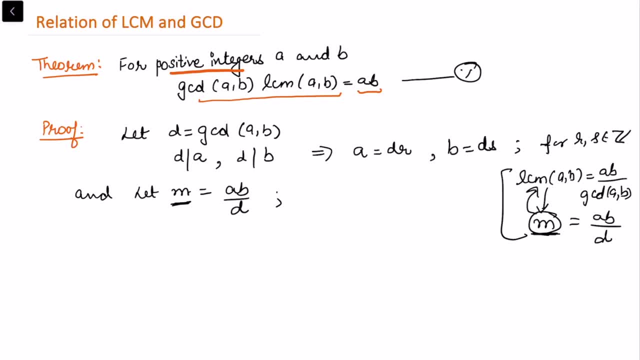 actually the lcm. So if m is the least common multiple, it must satisfy the definition of the least common multiple. In my last video I have talked about the definition of the least common multiple. So I have considered as least common multiple If a divide m and b divide m. this is 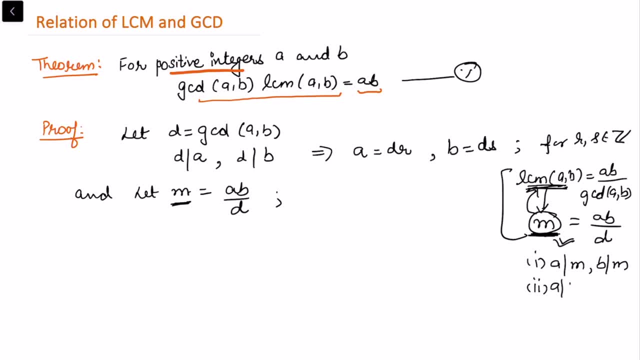 the first condition. Second condition is: whenever a divide c and b divide c, this m is always less than or equal to c. If these two condition are satisfied by this number m, then we say that m is acting as a gcd. Now what we have assumed is m, we have assumed as ab by d. So let us see. 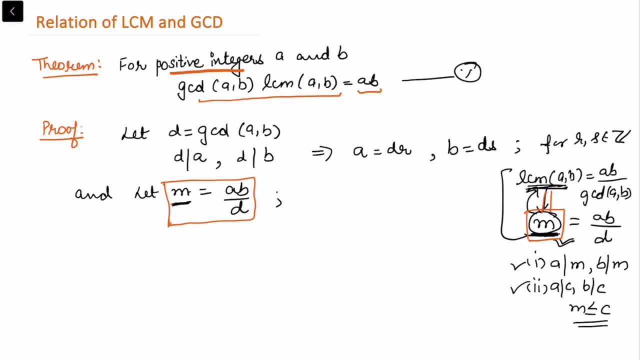 whether it satisfy the first condition or not. So, assuming that m is ab by d, So it is very that is also equal to rb. Just from this definition we can see that a by d is same as r, and from here b by d is equal to s. So now if you look at this expression, which is m is equal to ab. 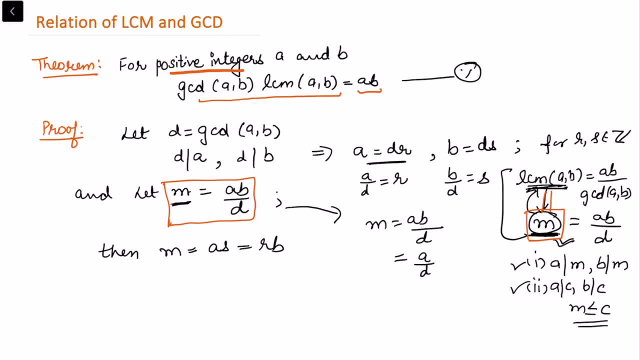 by d, So I can one time I can write this as ad multiply by. So if I write into this form. So this means ad is same as r and that is why r into b. So this will come if I write this expression. 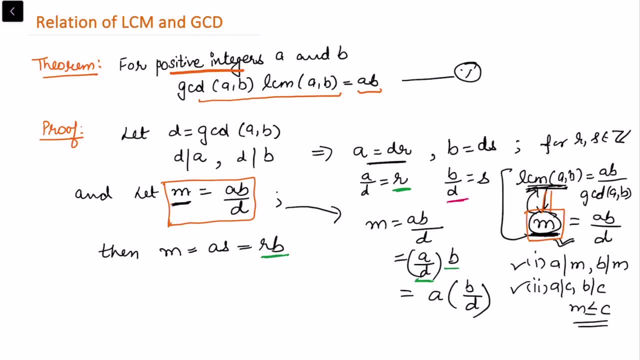 b by d. So in that case you can see that b by d is s and we can write it as a into s. So that is why I have written as, So whenever. so this means now, by looking at this condition, I can see that 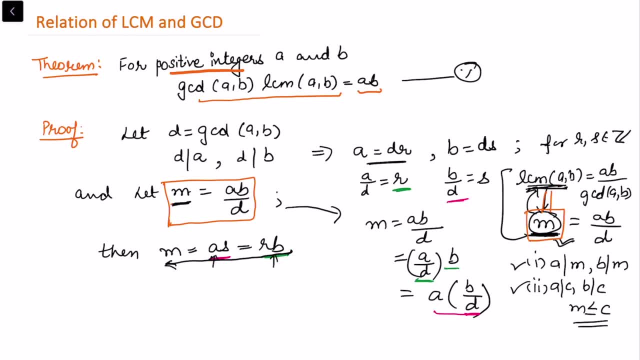 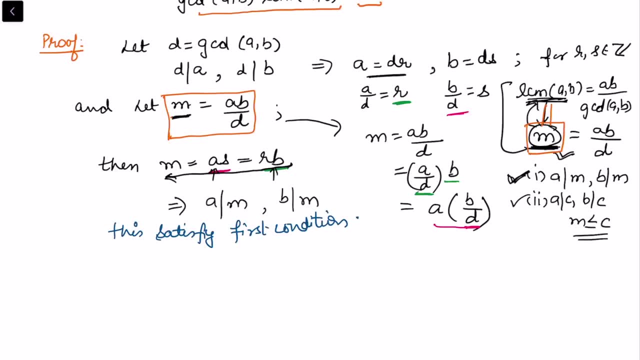 m is a multiple of a and m is a multiple of b, and from here you can see that a divides m and b divides m. So that satisfy the first condition. So we say this: satisfy first condition that m is a common multiple of a and b. So we write: m is a. 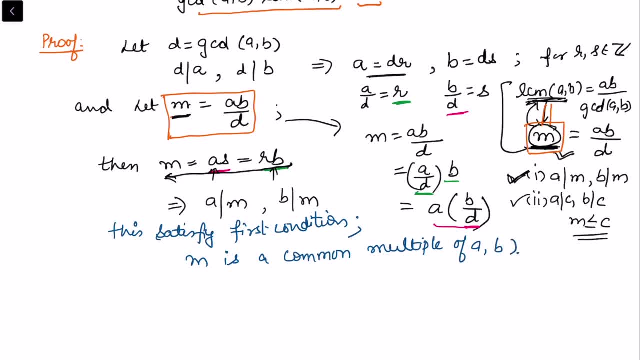 common multiple of a and b. So what we need to prove that it is not only common multiple but it is least common multiple. So for the least common multiple I also want to consider any other arbitrary integer. So let c be any positive integer that is common multiple of a and. 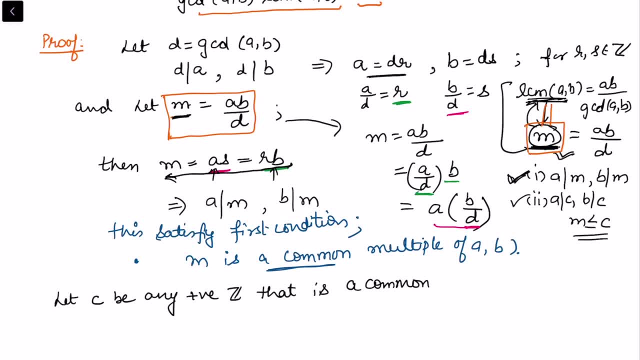 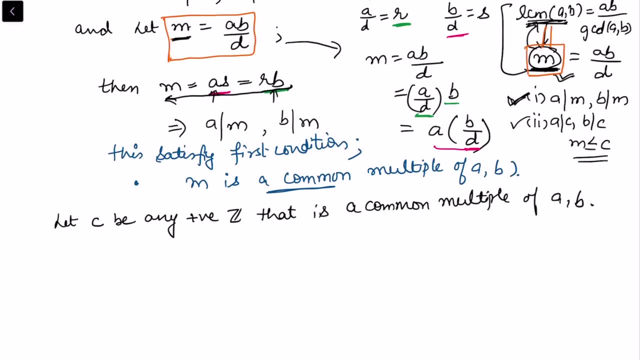 b. that is a common multiple of a and b. So let us consider now any other common multiple of a and b, and because now it is a common multiple of a and b, we can write that as a into s. So a common multiple of a and b. so obviously a divides c and b divides c and by definition i. 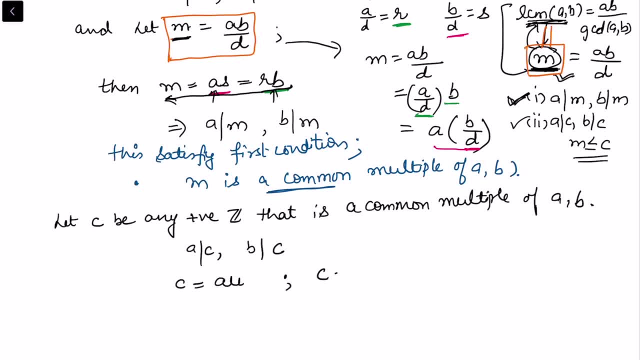 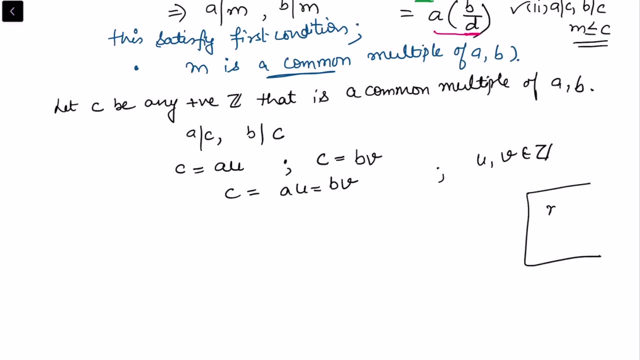 can write c as some au, and here i can write c as some bv. so, or we can simply write the c as u- au. that is same as bv for u and v belonging to integers. so for, and what now we need to prove? we need to prove that m is less than or equal to c. this is what we need to prove, and we note that. 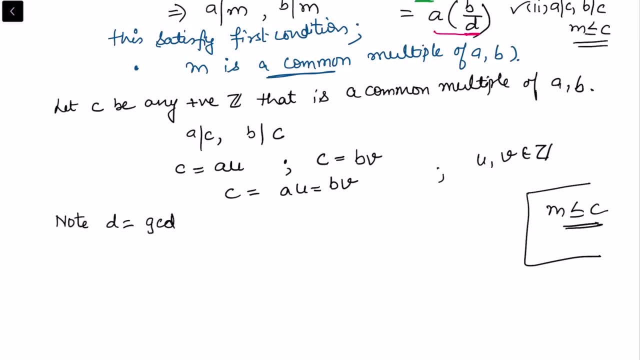 we have also considered d as a gcd of a and b. so d was considered as gcd of a and b and we also know that d- if i assume that d is gcd of a and b, i can write d as a linear combination of these two. for some x and y which belong to integer and that means, as a consequences of looking this, d, c and. 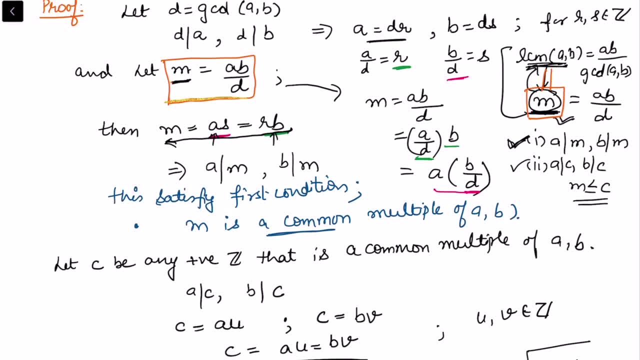 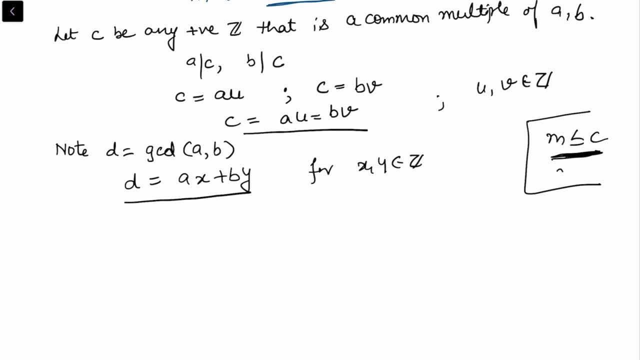 what is our expression for m? you note it down from here: m is ab by d. so now, just looking at this expression, and also because i want to show the m is less than or equal to c. so if i can show that m divides c. so now let's consider c by m. 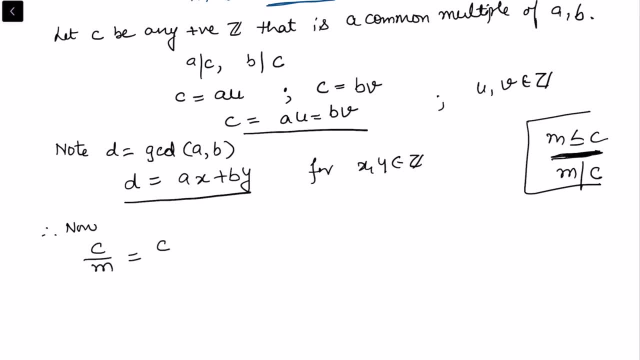 so i want to divide c by m. so that means this is same as cd by ab. so here i have simply substituted the value for m. the value for m that i've considered initially is ab by d. so that's just the substitution. and we know d is ax plus by, so this is ax plus by substitute here and this is ab. 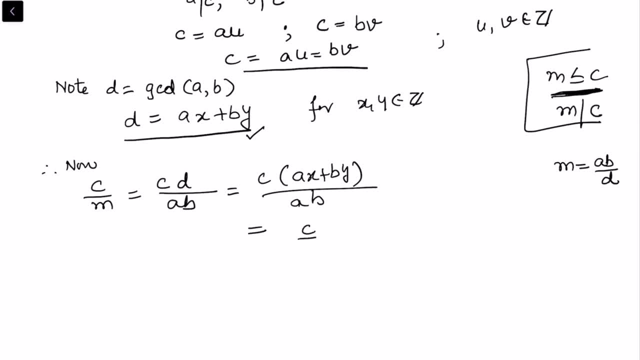 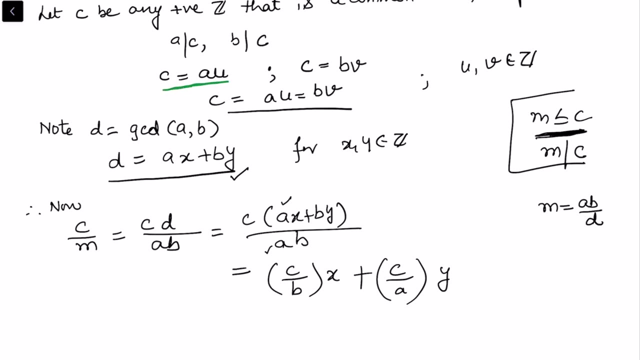 so now this becomes. so now just open it up. so this becomes c by a times x. from the first expression you can see that a and a will get cancelled. this will become c by b, plus the next term will give me c by a times y. now we have just assumed- look it back here. from this expression c is au and c. 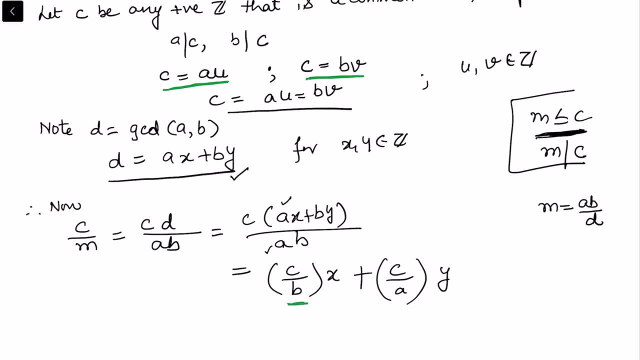 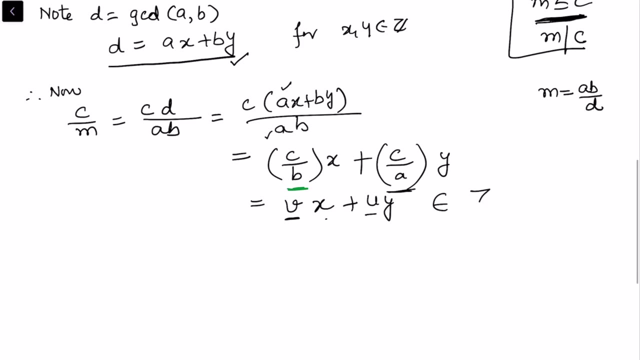 is bv. so when i take c by b, so this will give me. this will give me v times x from this, and when i take c by a, this will give me from here, this will give me u times y. now this is all integers: v u, x, y. they all integers. so this right hand side is an. 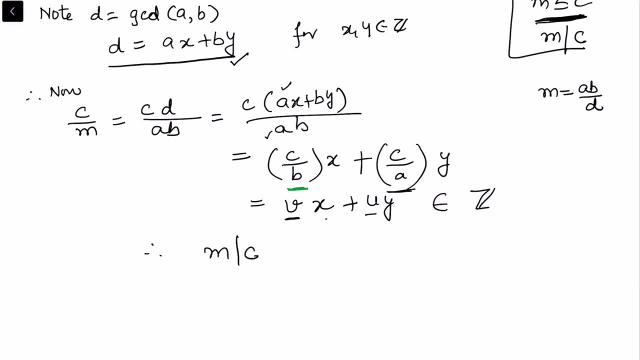 integer. so from here we can see that m divides c and this implies m must be less than or equal to c. so this satisfy the second condition. so this satisfy second condition, second condition of lcm. so this means that m is a common multiple as well as it's the least common. 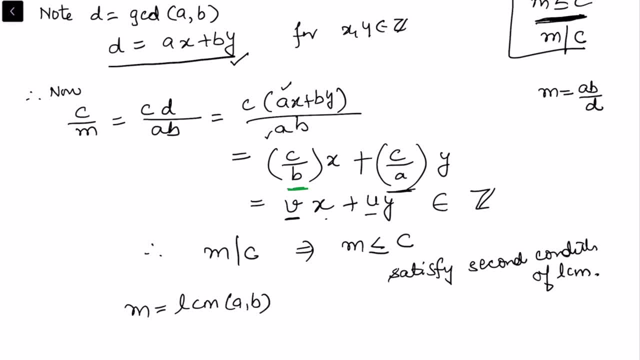 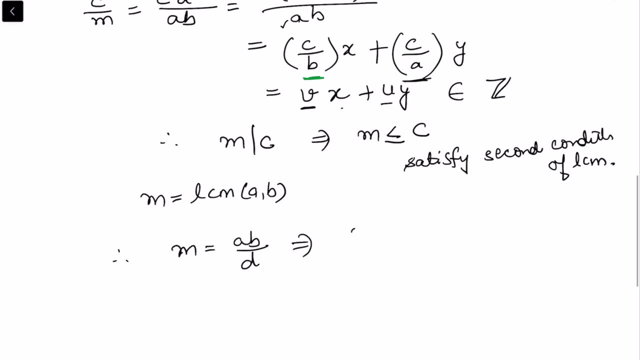 multiple. so m is least common multiple of a and b. and now, because m is the least common multiple, so we have assumed that m is ab by d. so from here this is: m multiplied by d is the product of the two integers. m we have taken as m we have proved as least common multiple of a and b, and d we have. 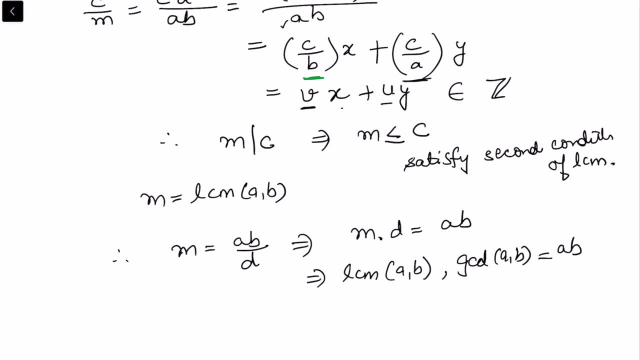 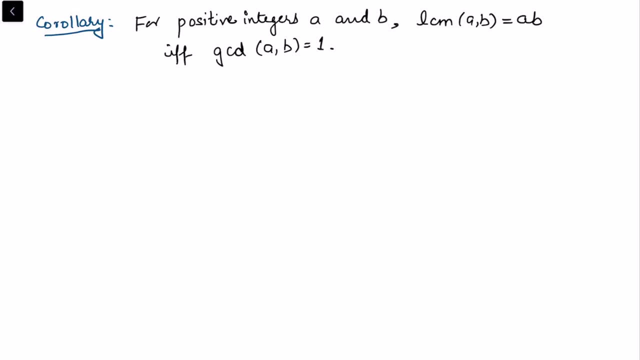 considered as gcd of a and b and that is equal to ab. and this is the expression that we desire to prove. and from the above this corollary is very obvious that for positive integer a and b least common multiple of a and b is the product a. 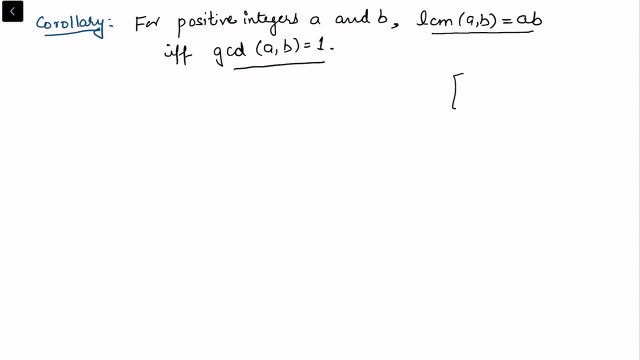 b if, and only if, gcd of a comma b is equal to one. so we have just seen that from the previous theorem, lcm of ab multiplied by gcd of a comma b, this is equal to the product of two positive integer. so whenever their gcd is one, that means these two integer, whenever they are relatively prime.